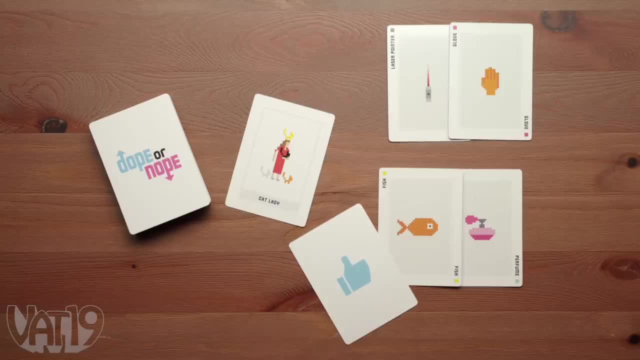 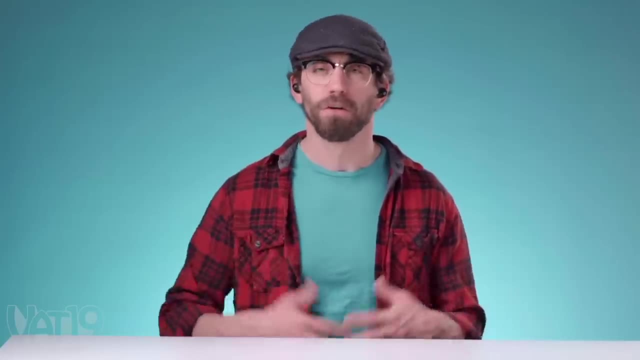 where you make combinations and there's a judge that gets to decide if they like your combinations. Can you give me an example of what some cards might be that you might acquire? Candy Couch, Candy Couch- Is that Dope or do you think that's Nope? 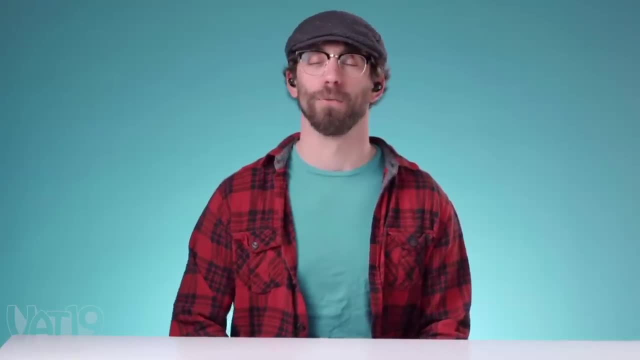 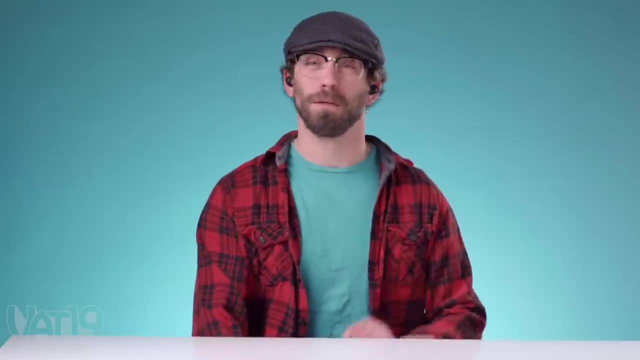 I mean, you could basically sit on your couch and eat your sorrows away and never have to leave. Yeah, I'd say that's pretty dope. Maybe we should actually watch some gameplay and see how it's actually played. Sounds like a plan. 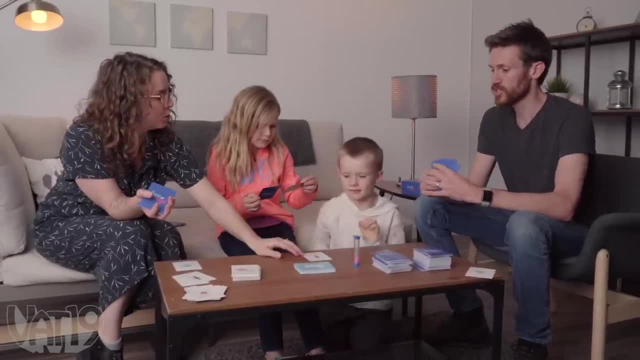 It is my turn to be the product. Okay, you a magician. What is a magician? A magician? Okay, so pick a product for a magician. James, sell me what you got. You have a hot dog and a hairspray. 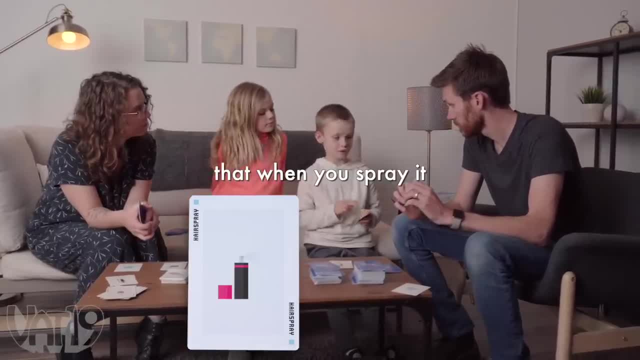 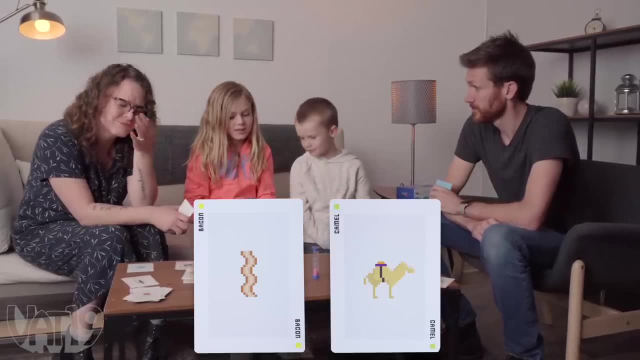 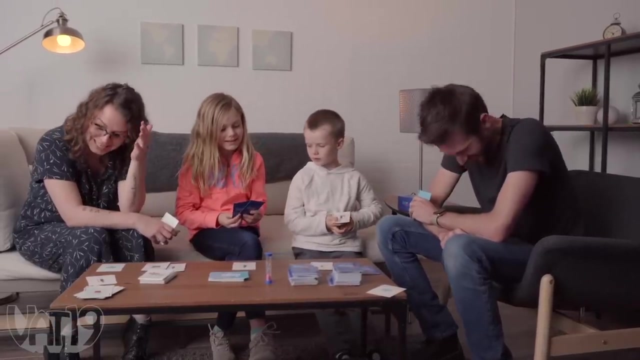 What is that? So it's a spray bottle that when you spray it it sprays out hot dogs. Okay, I have a, A bacon camel, So they can just bring a camel in and he'll eat some parts of the camel and it'll amaze. 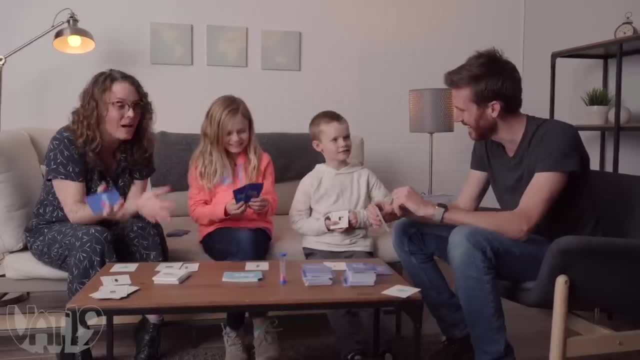 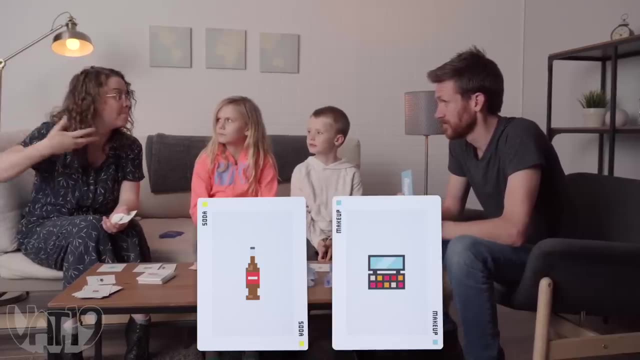 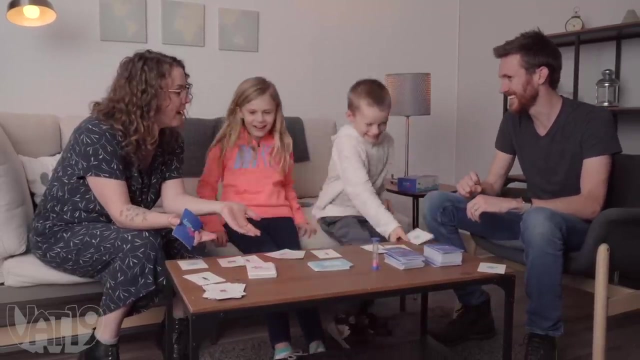 the crowd What My product is: a soda that when you pour it on yourself, it makes makeup appear. Spraying hot dogs is the closest to a magic trick. So, James, you have to go for the hot dog. No, it's soda makeup. 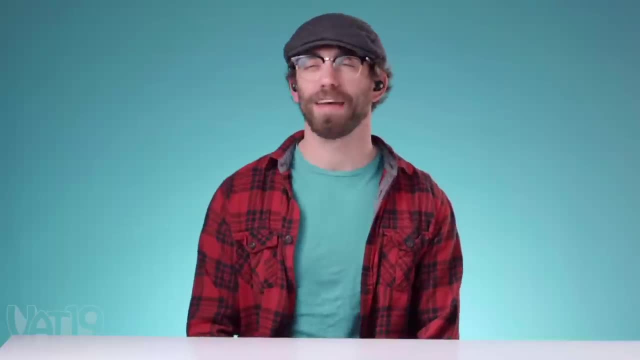 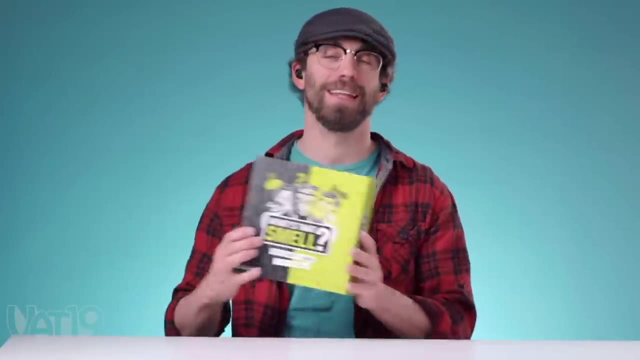 What are you talking about? Yes, yes, yes, yes, yes, yes. Sarah, I have a sense you're going to like this next game. Did you say sense or sense? I said sense, but it is. what is that smell? 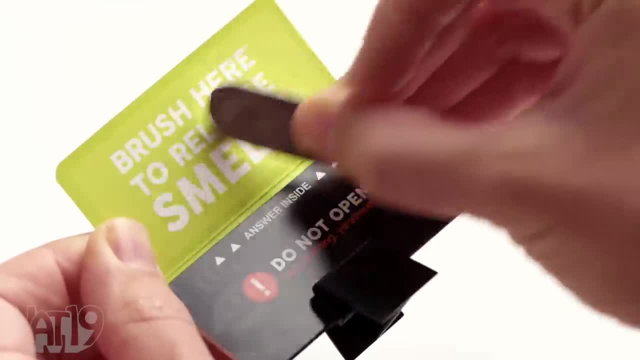 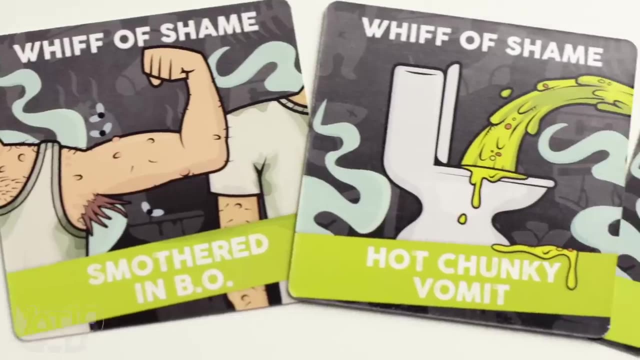 This is a game where you have to identify basically what the smell is. It's as simple as that. So it could be anything like a nice leather couch, or it could be like vomit, right, Right, Ooh, that smells like a fresh load of laundry. 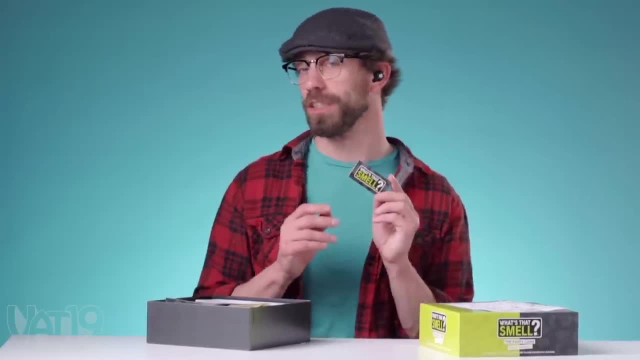 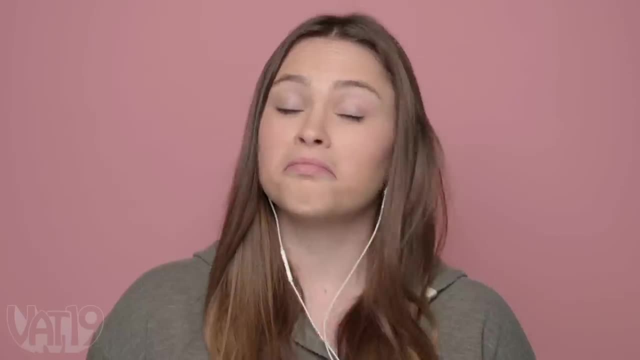 This might be a laundry detergent, Is it? Oh yeah, Did you get it right? It is detergent. as you can see, I got it right. Five points. if you get it right, Three points for anything close, So like fresh laundry or soap, would be close. 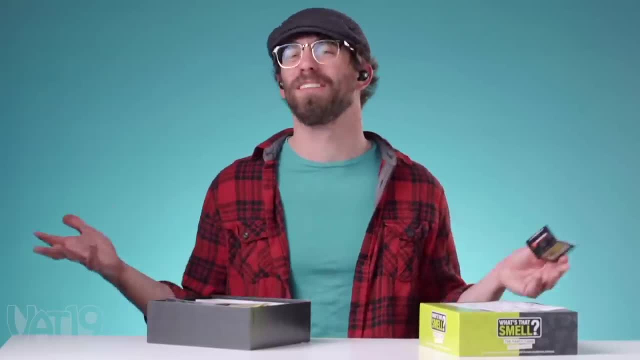 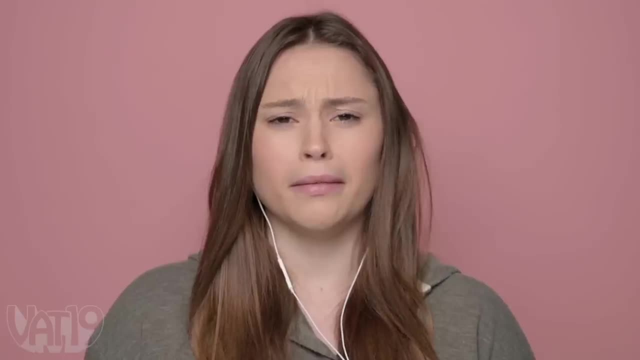 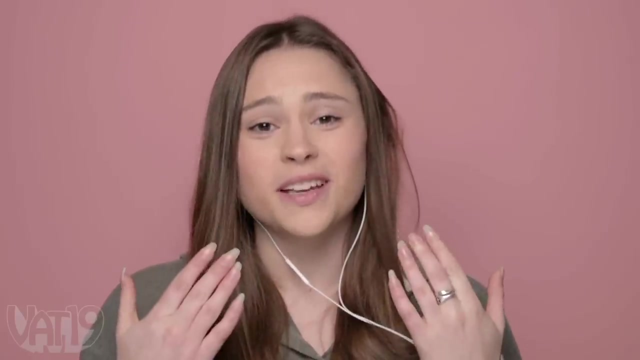 And one point: if it's something in the category, So all things chemical would work for that, You also get whiff of shames, like this smothered MBO card right here which smells like somebody did not take a shower. Well, my sniffer is pretty sensitive. 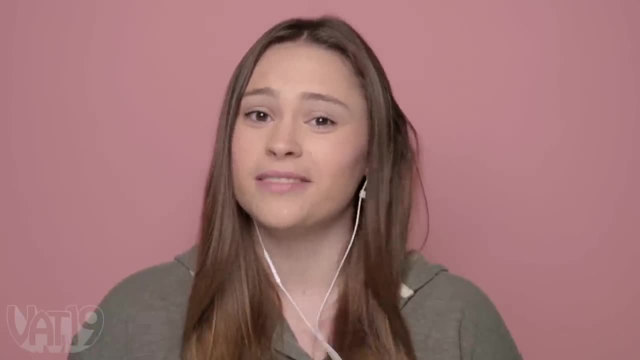 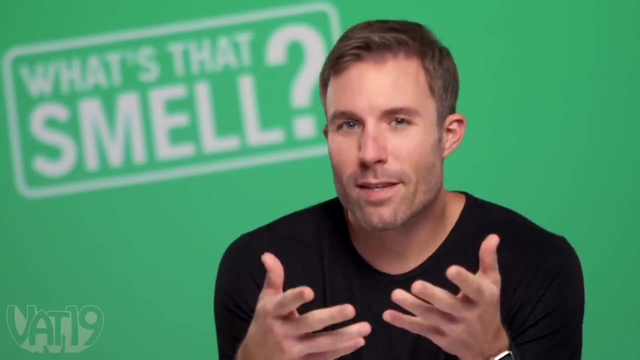 So I'm really glad we don't have to play this game. Let's watch somebody else play it. Yeah, You're so quick, Very confident. I know what this is, but I'm not sure what they're going to say it is: 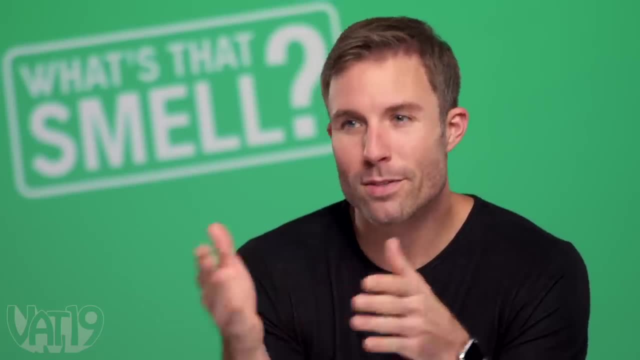 I think it's a spice that goes in something, But is it the something they want or is it the spice? Oh, I know that smell, but I can't think of it- Some kind of spice that I've used in the kitchen. 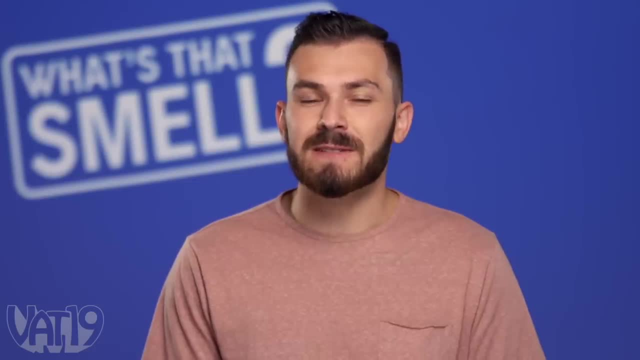 Gosh, I know what that is. I'm just going to be super general and put down spices, And hopefully I'll get some kind of umbrella point for that. This one's definitely cumin, but cumin is one of the main ingredients. 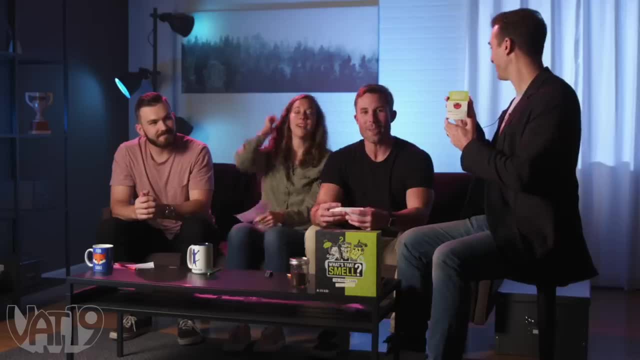 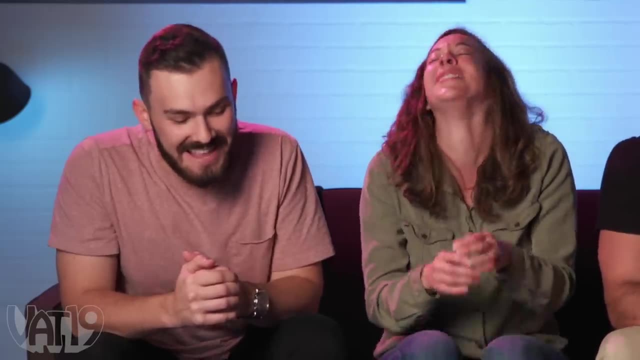 And chili. So is it chili. Did anyone say chili? Oh yeah, Chili powder. Chili, It just says chili. I'd accept chili powder Once again. I have lost. I just wrote spices because I couldn't think of the specific spice that it smelled like. 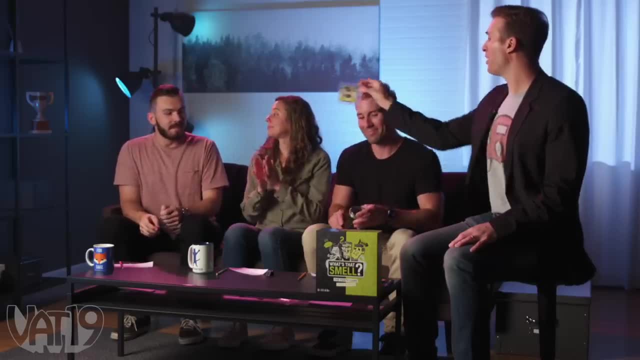 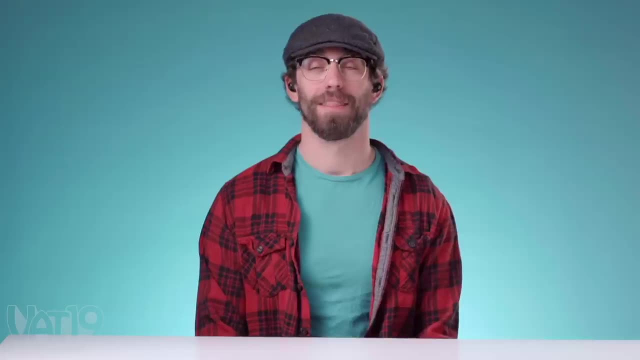 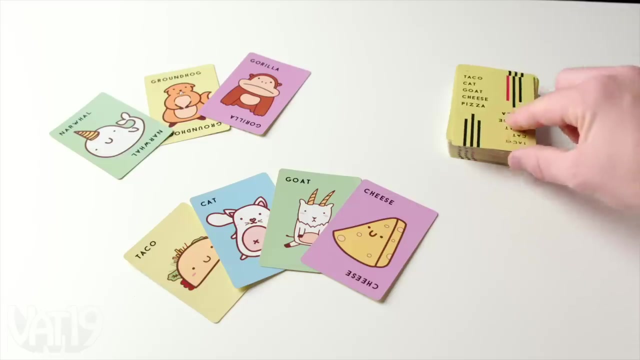 OK, Drew, smothered in BO is your punishment. That smells like a zoo exhibit. That is terrible. Well, that game stinks, but in a good way. That pun was stinky, I thought it was sweet, But if you want a game that has a lot less rules and is a lot more frantic, we have Taco. 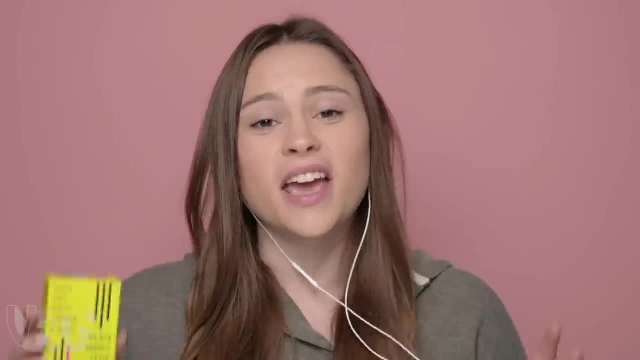 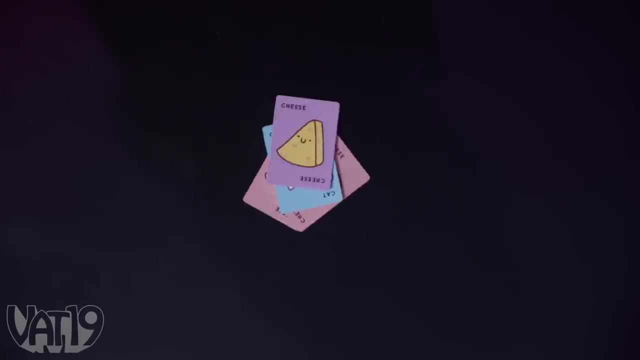 Cat Goat Cheese Pizza. This game is insane. It's a huge brain buster where you have to say taco, cat goat cheese and pizza, all in order, while laying down a card. If you happen to say the word that matches up with your card, you've got to smack that. 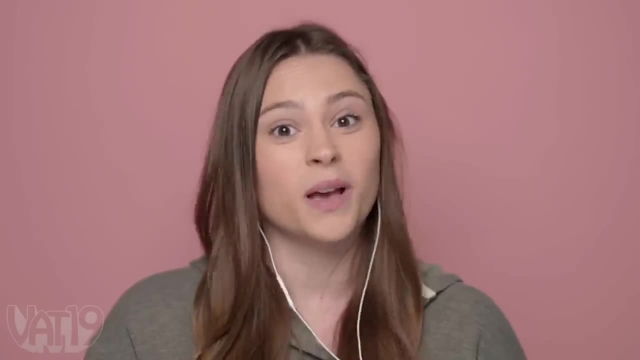 card And the last person to smack the deck. well, they've got to pick up the pile And your goal is to get rid of all of your cards, so you don't want to be the last person to slap that pile, Sarah. 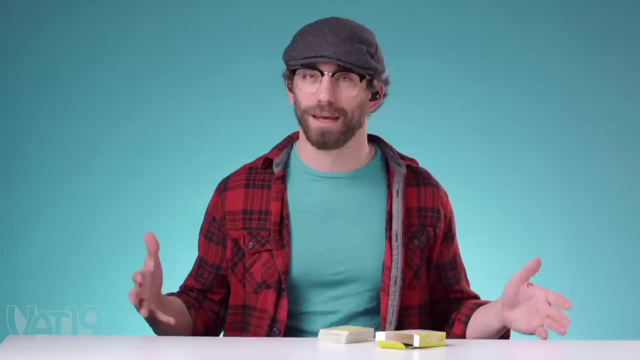 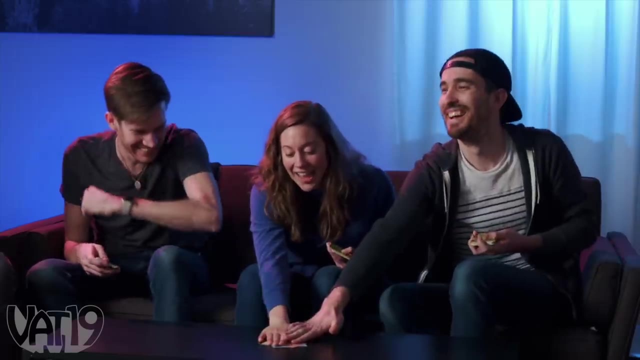 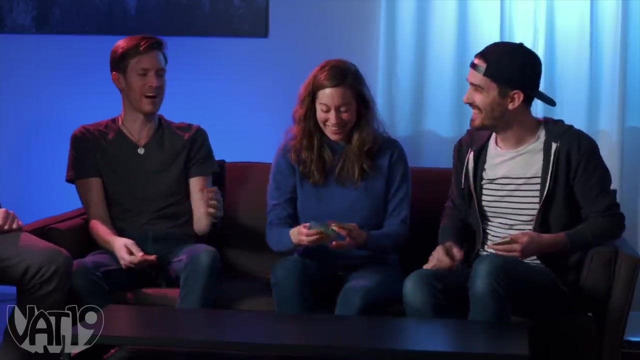 Probably the best way to see and understand this game is to just play it, because it's way more fun. So let's watch it in action. Taco Cat- Goat Cheese Kara's speedy Taco Cat. Sometimes you just watch it happen like, well, all right. 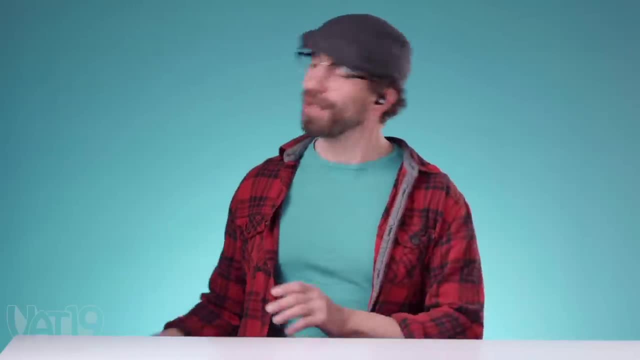 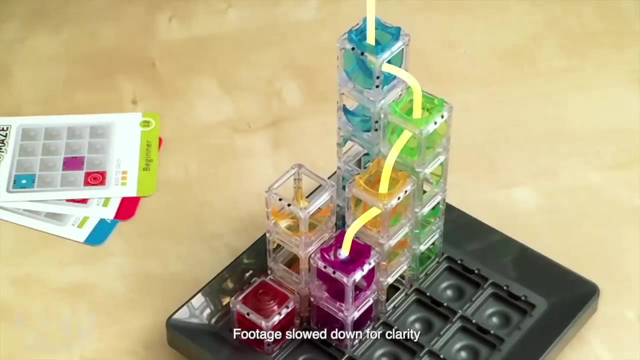 Sarah, if you're in the mood for more of a solo thinking game, I'd recommend Gravity Maze. Gravity Maze- Oh, I love that one. It's like you have this marble and you have to get it from a place- Point A to B, using all sorts of different columns, making it go forwards and backwards. 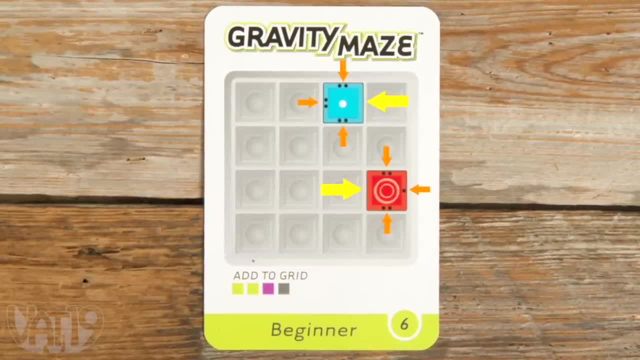 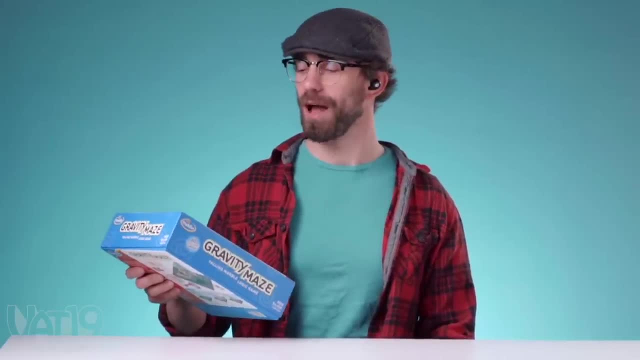 and up and down. There's 60 different challenges, anywhere from easy to expert, And I really want to see you play it. Adam, You know what I kind of like- logic games- so why don't I just unbox this and give it a shot? 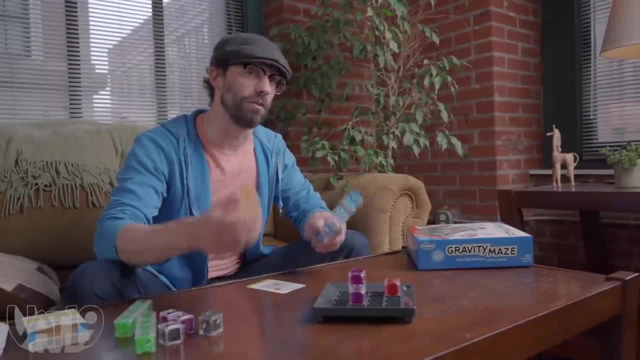 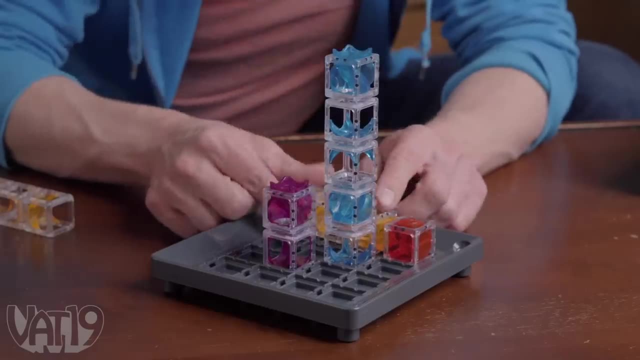 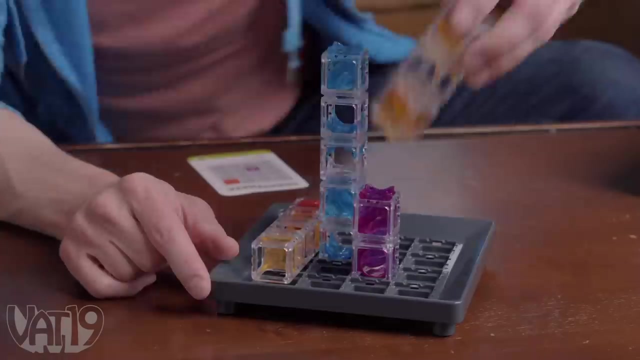 So I have to incorporate a blue and two yellows to make my marble run through this maze. I have to start here and get to here. Maybe I can do a piece like That running like that. Do I have it figured out? I don't know. 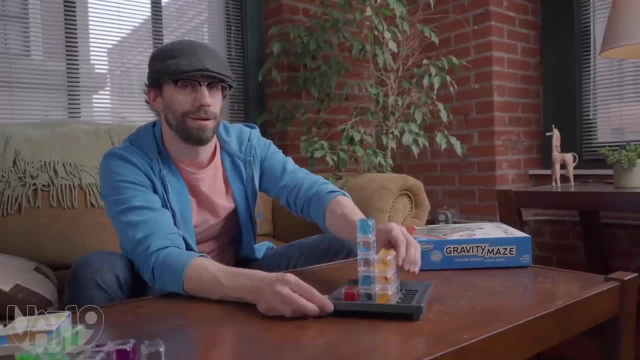 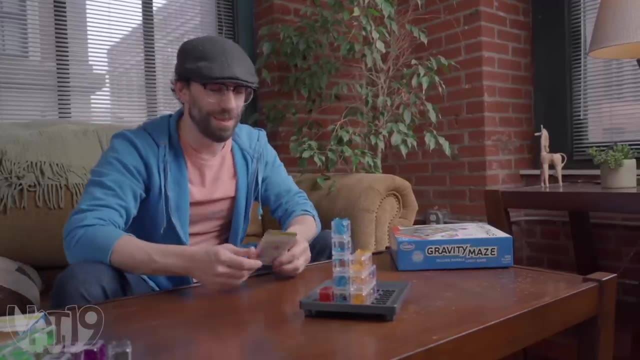 Maybe if I stack that there and I think I'm good to go, Let's find out. It's pretty good See, if that's the answer. That is in fact the answer I can do, a beginner one. So yeah, that's Gravity Maze. 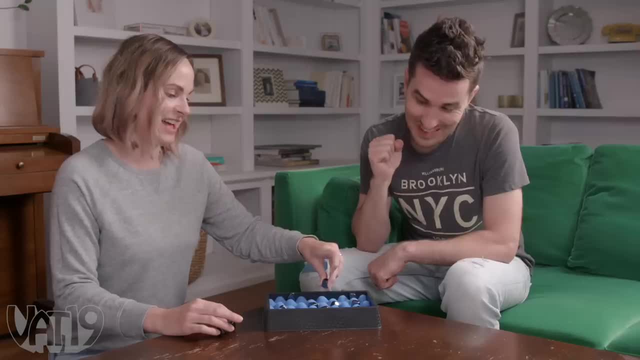 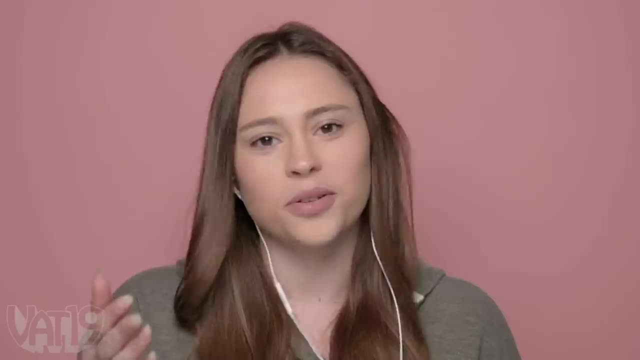 It's pretty cool. We've got Jishaku up next. This game has all of the things you need for a game of skill. It's got magnets- all the things that I know you care about so deeply. I love all of this. 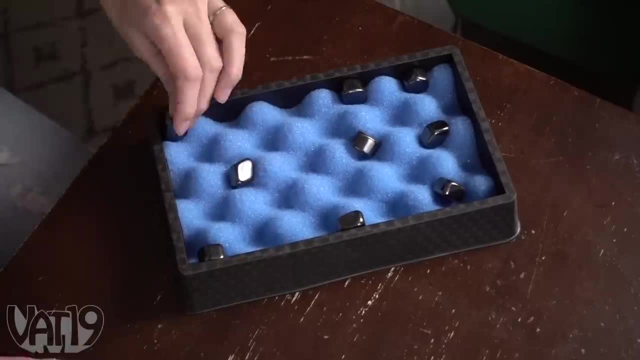 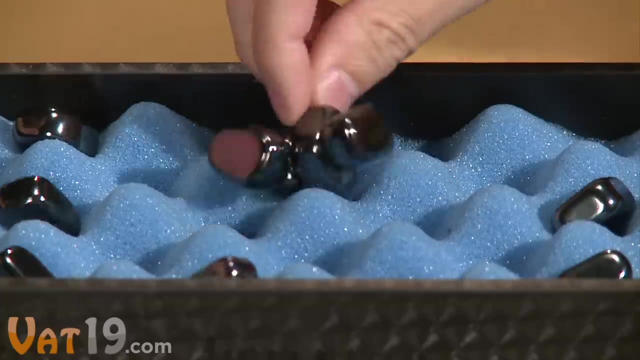 Yeah, Really you have 18 magnets that you're trying to fit into the little divots on the board. But you have to be careful with the polarity. So if you've got two magnets close to each other and they touch, you lose. 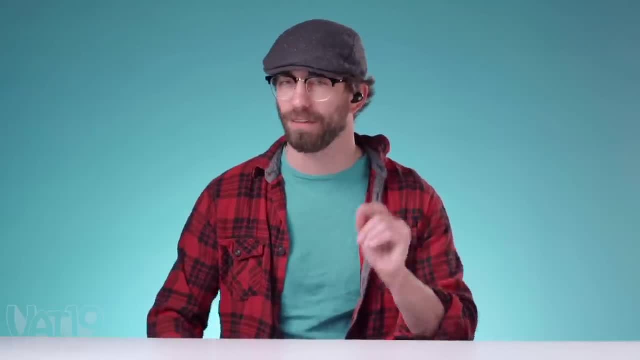 So you've got to be really, really careful with how you're placing your pieces. Well, Adam, since we're here, we're going to go ahead and get started. Since you're the master of magnetism, I'll throw this one to you. 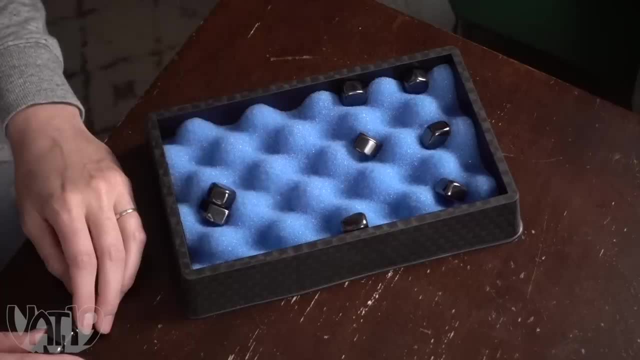 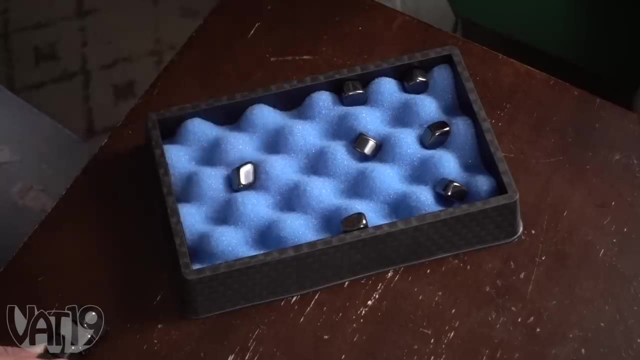 Let's go check it out. I'm going to put it right here. Oh, dang it, You shouldn't have been so cocky. I was really cocky. All right, I'll take these. These are mine. Yeah, good move. 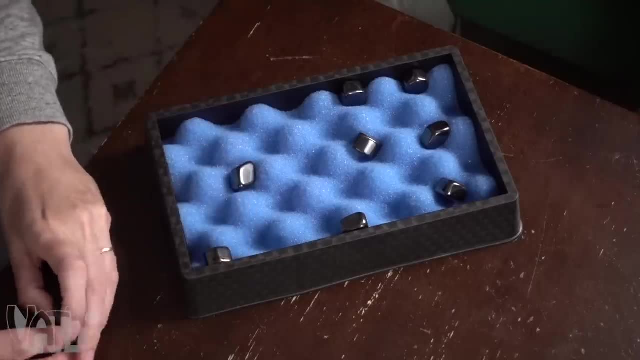 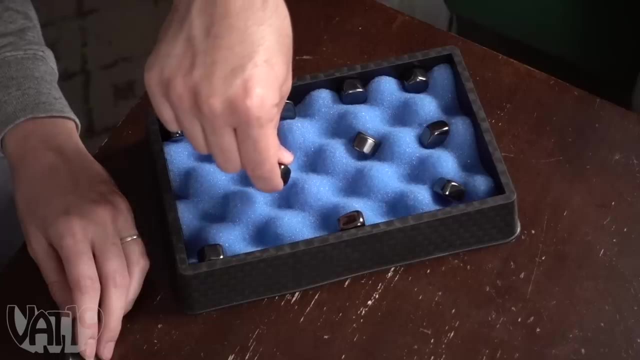 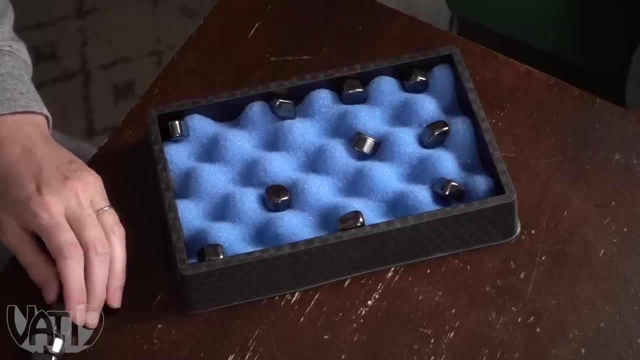 All right, I'm going to go cowardly. Classic corners. This is probably the game-winning drop right here. Can't get too cocky, All right, Oh It's in, You can be doing so well. and then It seems like it should be easy. 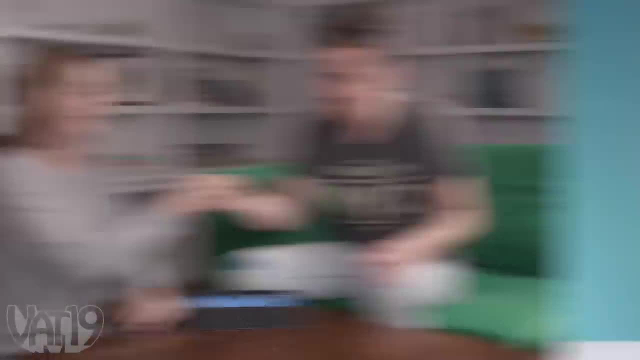 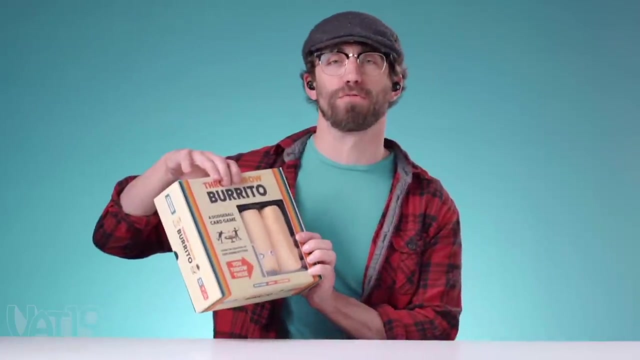 It's really tricky, It's really hard. Good game, Sarah. if you're looking for a little bit of collision with your gameplay, then I've got the game for you. Throw Throw Burrito. Oh, I love this game. It's basically dodgeball meets card game. 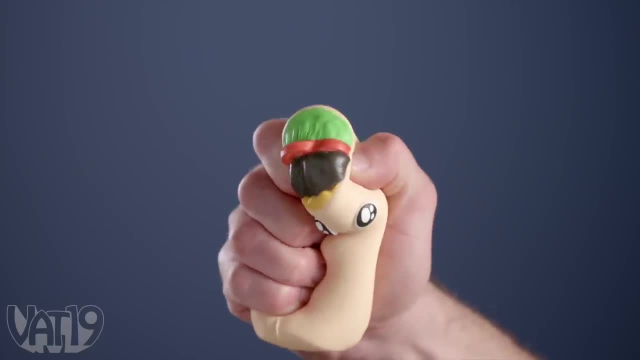 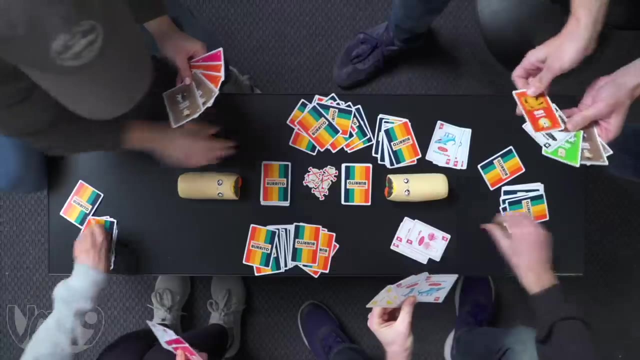 It's pretty sweet. You've got these squishy foam dodgeball burrito things here. It's like a card game where you have to get three of a kind And if you match any of these interesting cards like three burrito brawls in your set of cards. 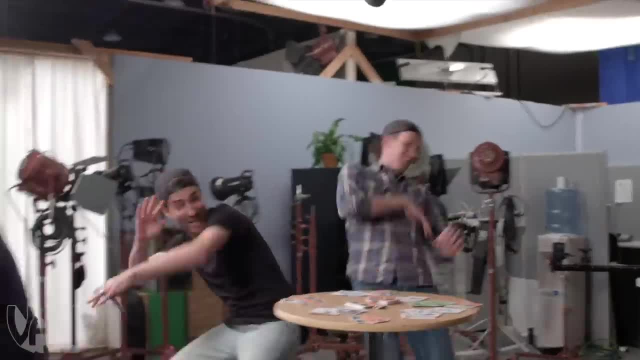 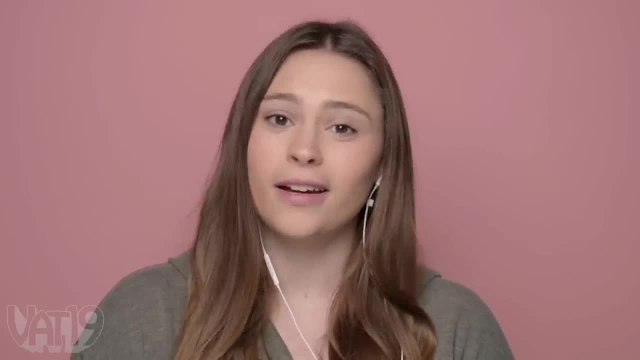 you have to do a little burrito brawl with your opposing player, And these little dodgeball burritos are not painful. I would know I chucked one at your face for the product shot and you were just fine. So let's throw to that gameplay. 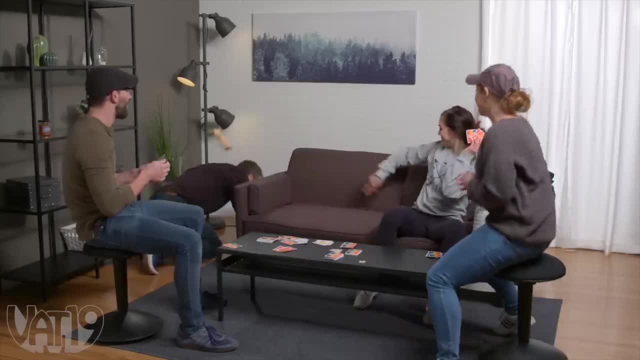 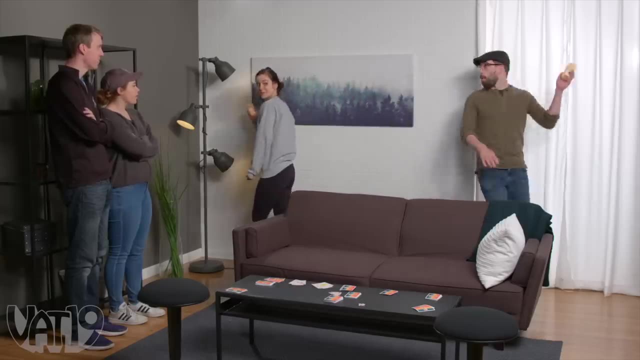 In a war everyone else goes to war. It's every man for himself and it can get pretty crazy. For a burrito duel. you get to pick any two players and have them fight And have them walk three paces and turn to fire. 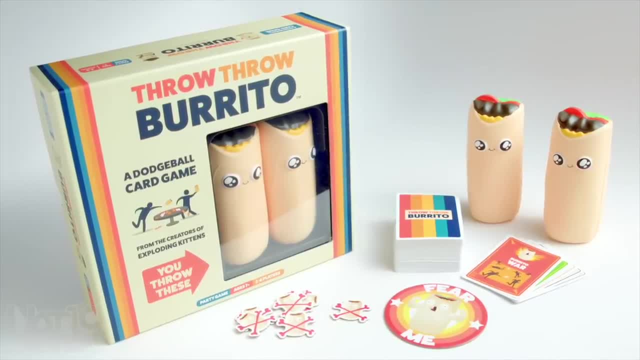 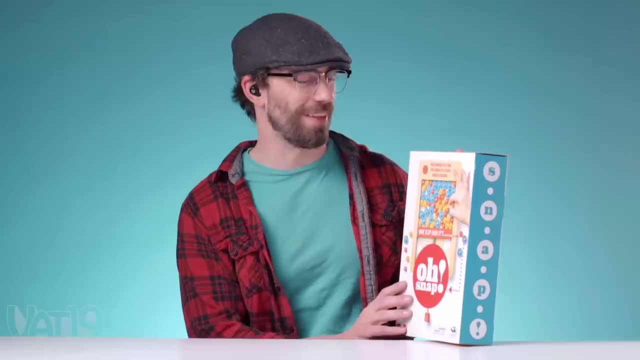 So get ready for a heated game of Throw, Throw. Burrito Three, two, one burrito. Oh snap, Adam, Check out our next game. This game is a lot of fun. It's pretty intense. Basically, what you're doing is you're. 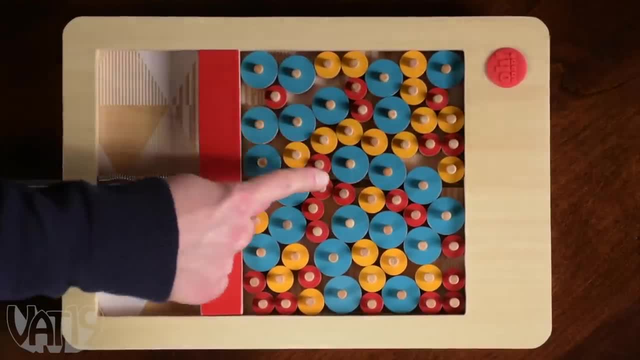 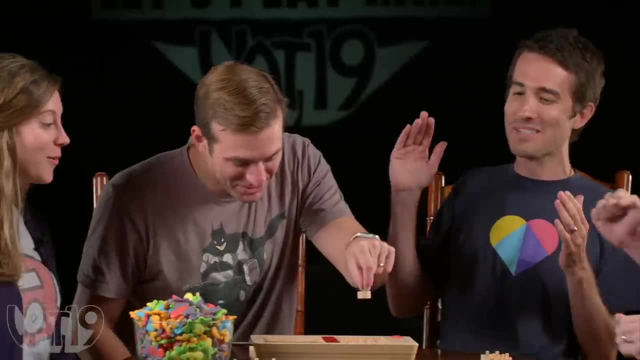 pulling different colored pieces out which are all worth different points, And you have this tension bar right here that if you pull the wrong piece out, will cause it to snap And you'll lose the game. just like that. The game's kind of like Jango, where. 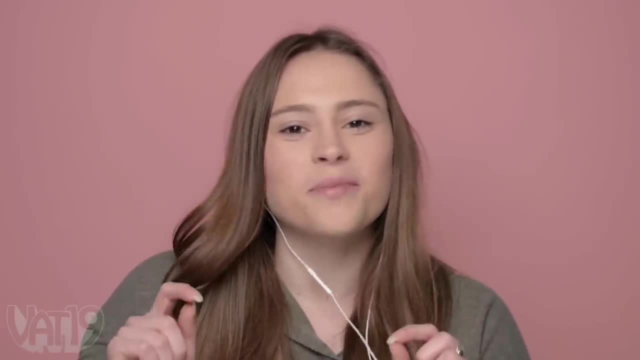 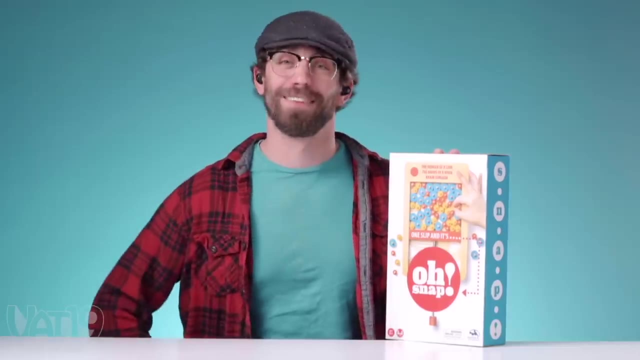 you have to pull specific pieces at very strategic times to make sure that it all doesn't come crashing down or, I guess, snapping up. in this case, It's a lot of fun. Yeah, let's take a look. I think this one right here is coming out. 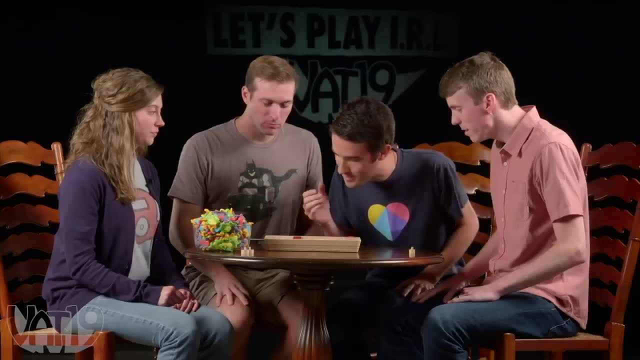 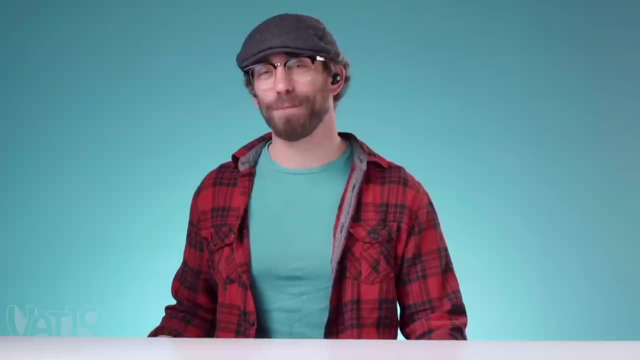 Oh, dang it What. I'll try it, but this is probably going to move it. That snap sound is just ah. Next up, Sarah, I've got a favorite game of mine. This is Happy Salmon, So everybody has a set of cards that they call out. 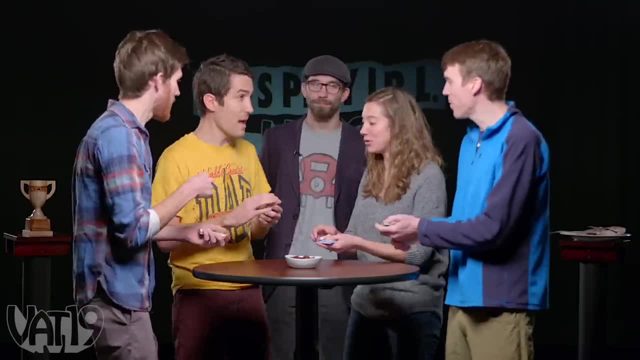 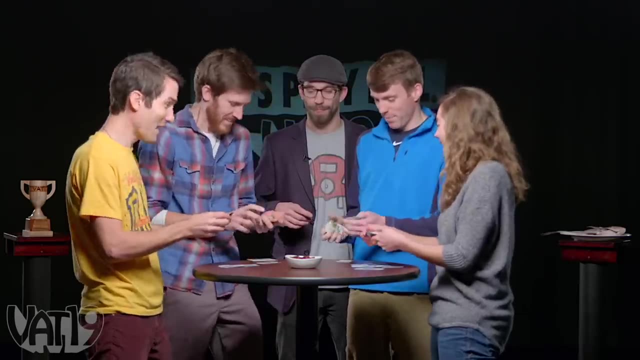 the actions on their cards And if they're able to get those actions like a high five, then they get to drop their card and keep going. So you can get a high five, a pound, a switcheroo or a happy salmon, which kind of looks like that. 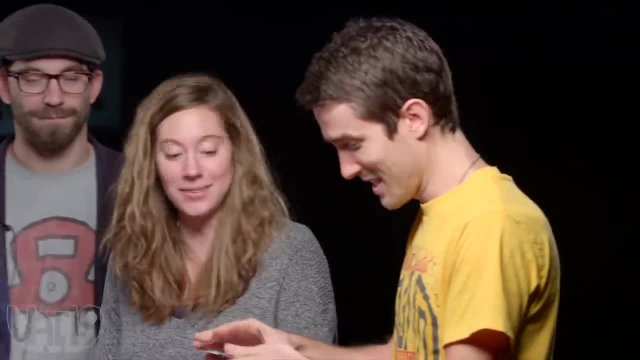 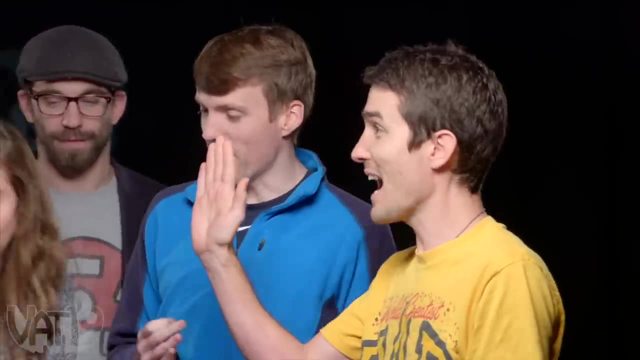 Now, the fun thing about this game is everybody is trying to get a match with somebody else, So there's a lot of calling out and a lot of yelling involved. while everybody's trying to get their own match, There's a lot of high fives that go un-high fived. 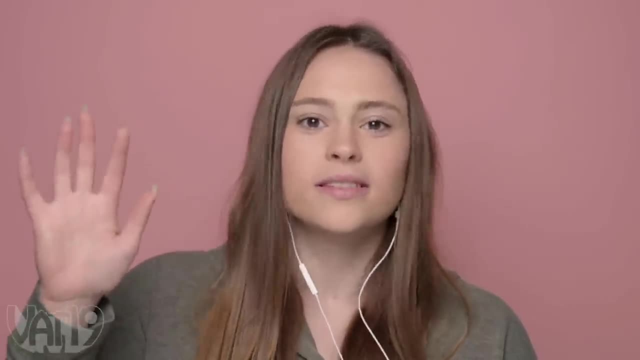 You just kind of stand there, You 15 seconds, any of your guard over and you're having an issue. So I think this race is going to win. I think you guys are going to win. I think you're going to win. I think you're going to win.